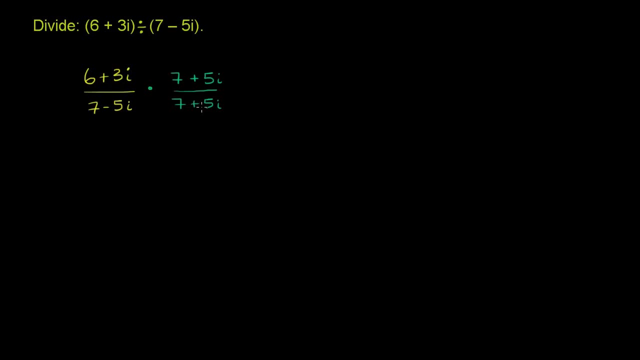 And anything divided by itself is going to be 1, assuming that you're not dealing with 0.. 0 over 0 is undefined, But 7 plus 5i over 7 plus 5i is 1.. So we're not changing the value of this. 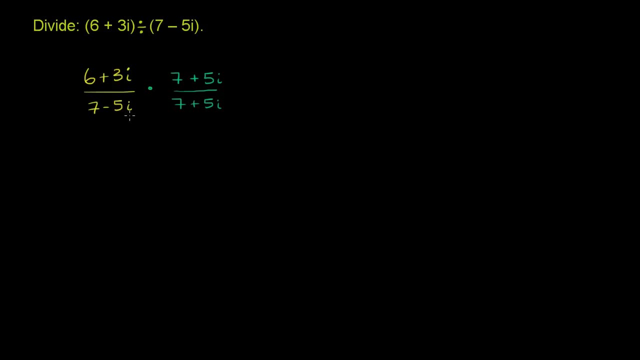 But what this does is it allows us to get rid of the imaginary number, The imaginary part in the denominator. So let's multiply this out, Our numerator. we just have to multiply every part of this complex number times every part of this complex number. 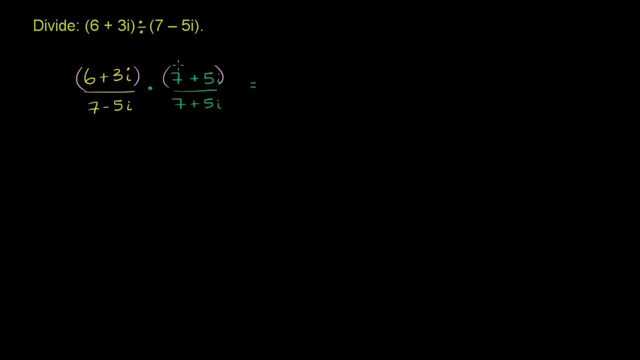 You can think of it as FOIL, if you like. We're really just doing the distributive property twice. We have 6 times 7,, which is 42. And then we have 6 times 5i, which is 30i. 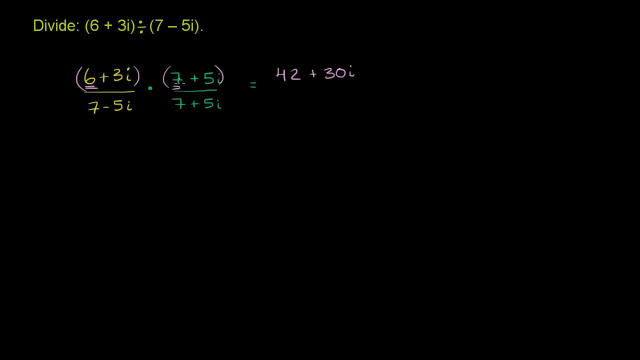 plus 30i, And then we have 3i times 7.. So that's plus 21i. And then, finally, we have 3i times 5i. 3 times 5 is 15.. But we have i times i, or i squared, which is negative 1.. 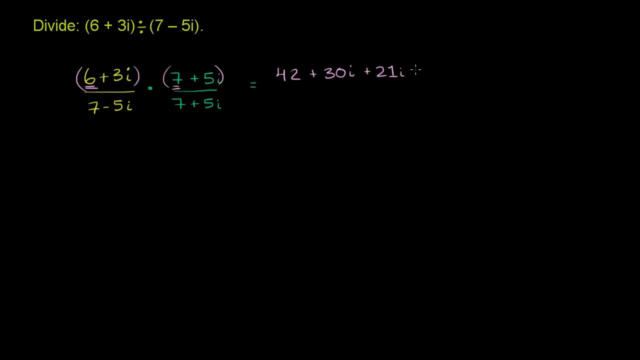 So it would be 15 times negative 1, or minus 15.. So that's our numerator And then our denominator is going to be 15.. OK, So we have a plus b times a minus b. You could think of it that way. 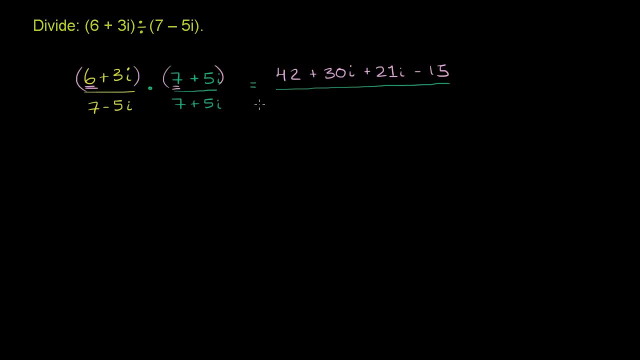 Or you could just do what we just did up here. Actually, let's just do what we did up here so you don't have to remember that difference of squares pattern and all of that, 7 times 7 is 49.. Let's think of it in a FOIL way if that is helpful for you. 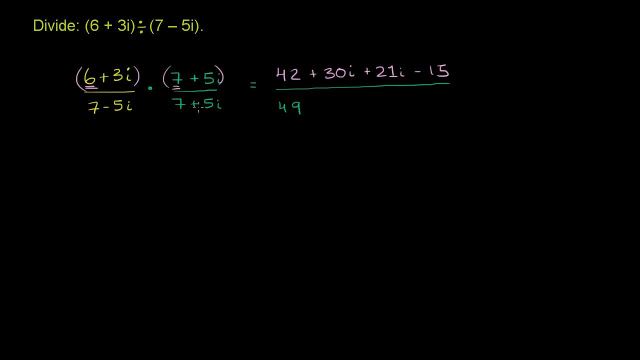 So first we did the 7 times a 7.. Then we could do the outer terms: 7 times 5i is plus 35i. Then we could do the inner terms Negative: 5i times 7 is minus 35i. 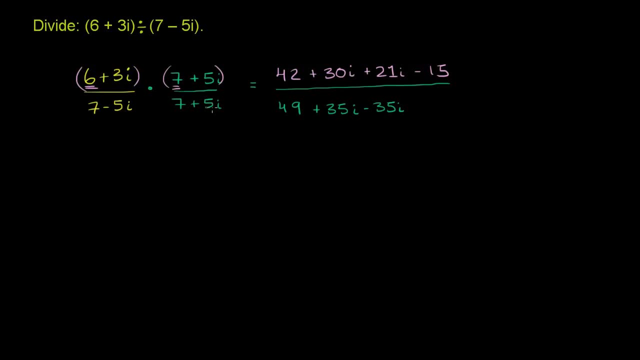 These two are going to cancel out. And then negative 5i times 5i is negative 25i squared. Negative 25i squared is the same thing as negative 25 times negative 1. So that is plus 25.. Now let's simplify them.